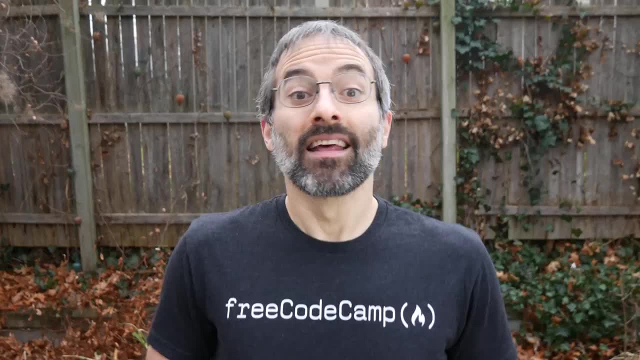 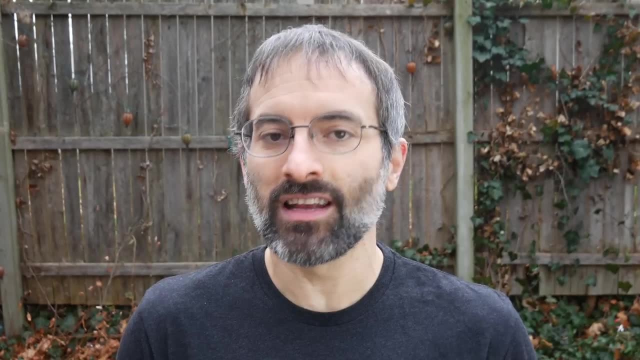 become a back-end developer, this is where to start. This is our Back-end Developer Roadmap. We've curated a collection of top-notch courses on all the key technologies you need to learn, and you can watch them right here on our channel for free. 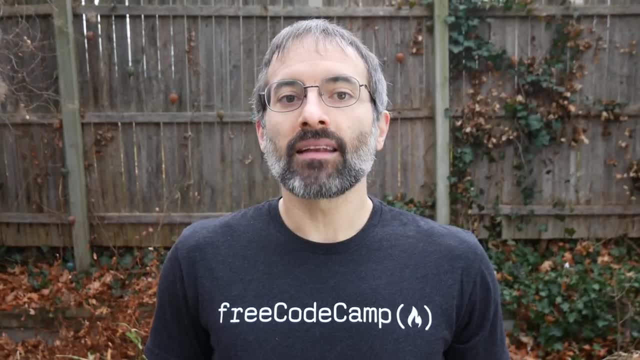 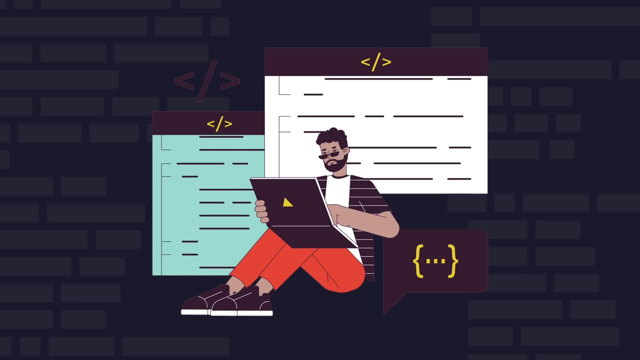 So let's start by defining what back-end development is. A back-end developer is a type of programmer who focuses on creating the underlying logic and server-side software that powers web-based technology websites and applications. Their primary responsibilities include server-side logic. 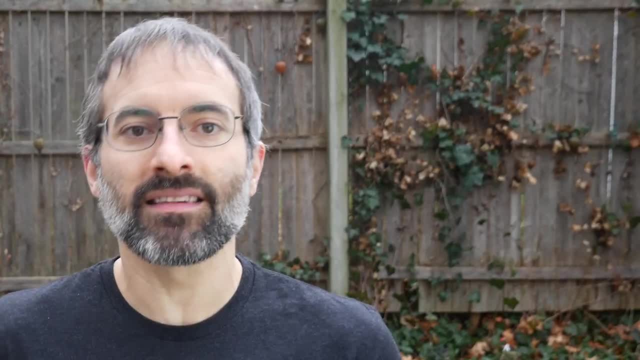 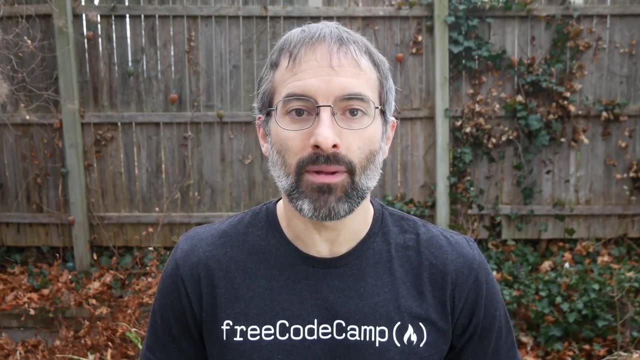 They write the code that runs on web servers, which handles the business logic of an application. This includes processing user requests, interacting with databases and controlling the flow of data between the server and the front end of the website or application: Database management. 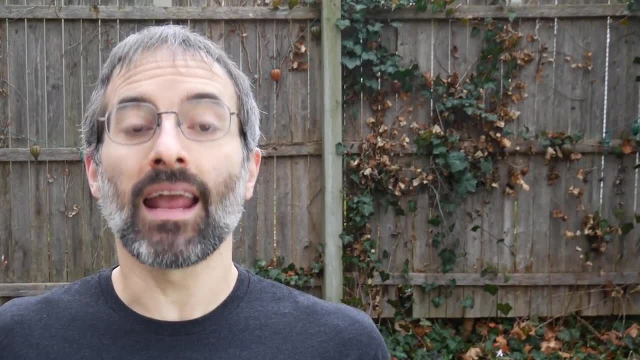 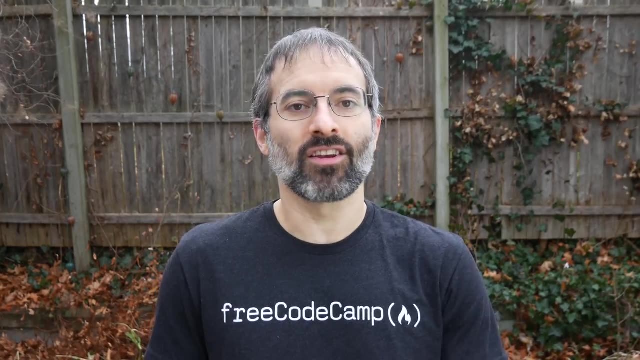 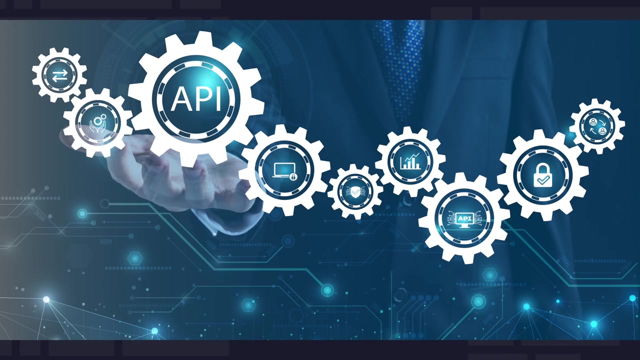 Back-end developers are often responsible for designing, implementing and maintaining databases. They manage and manipulate the data that's stored in these databases, ensuring its integrity and security. API development: They often create Application Programming Interfaces or APIs, which allow different software applications to communicate with each other. These APIs are crucial for the integration of different systems and for enabling front-end applications to access server-side functions and data Server management. They may also be involved in configuring and managing the servers where the applications run. This can include setting up cloud-based servers. 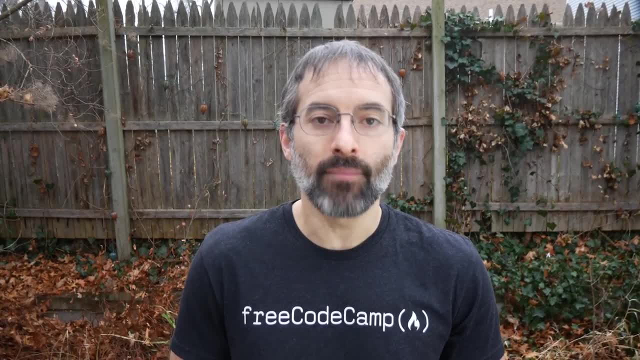 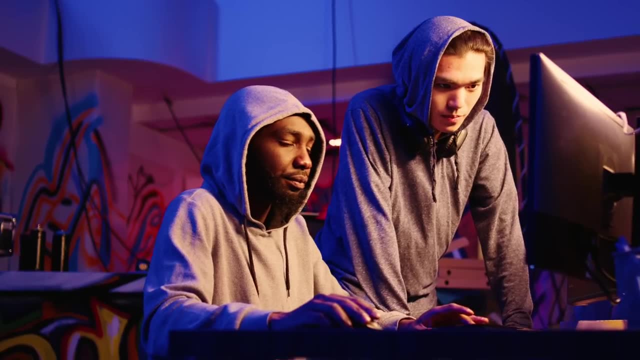 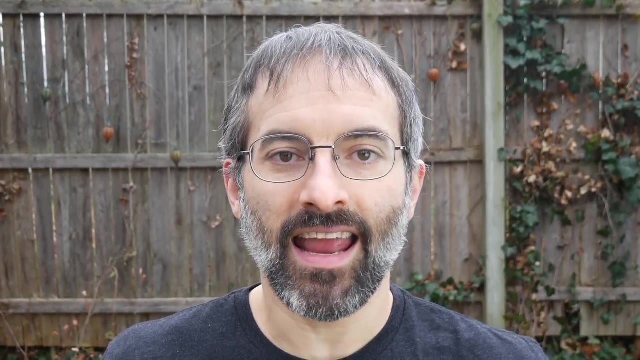 Managing server resources and securing uptime and performance Security. Ensuring the security of the web application is a key part of a back-end developer's job. This includes protecting against various types of cyber threats, securing data and implementing authentication and authorization schemes. 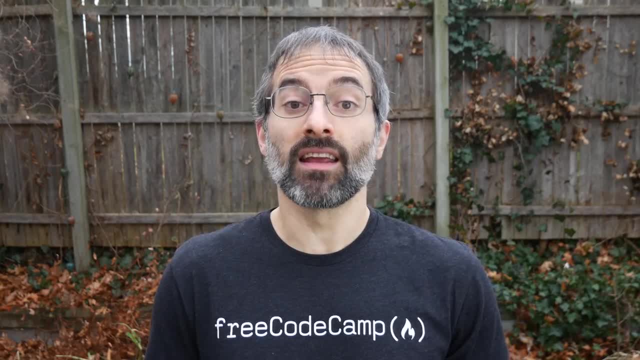 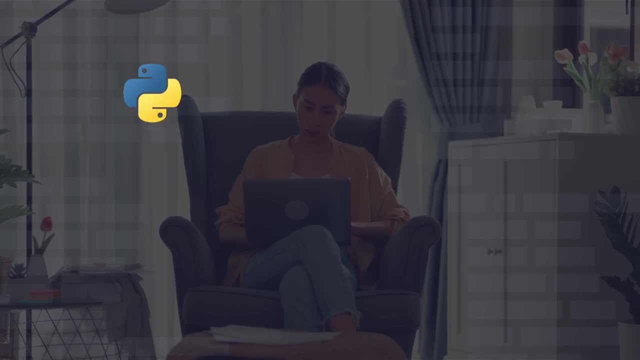 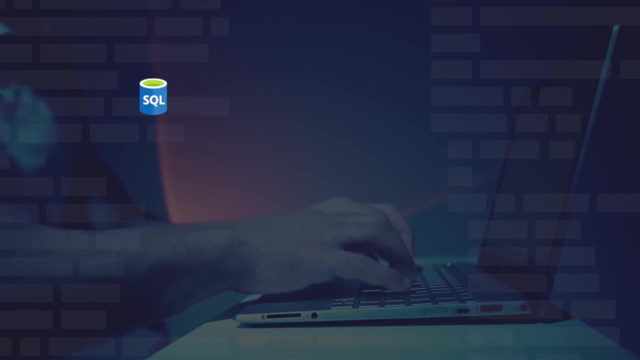 Becoming a back-end developer typically begins with acquiring a strong foundation in computer science. The core of this learning journey involves mastering server-side programming languages such as Python, Java, JavaScript, Nodejs and NET, and getting expertise in database management with systems like SQL, MySQL, PostgreSQL or MongoDB. Additionally, familiarity with server management, cloud services and containerization technologies is increasingly important. Practical skills can be further developed through personal projects, internships or contributing to open-source projects, Continuously learning, Learning and staying updated with all the latest technological trends, as well as engaging. 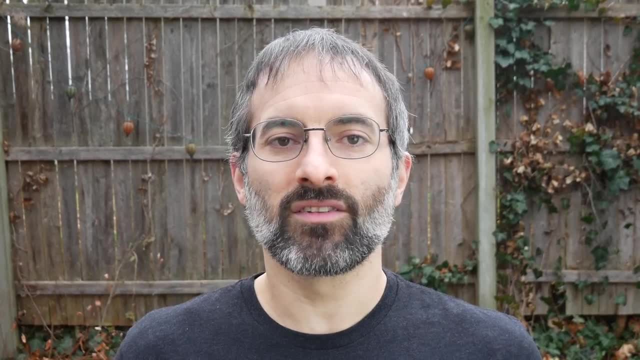 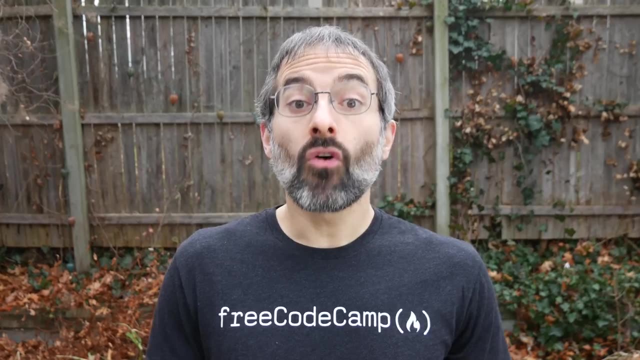 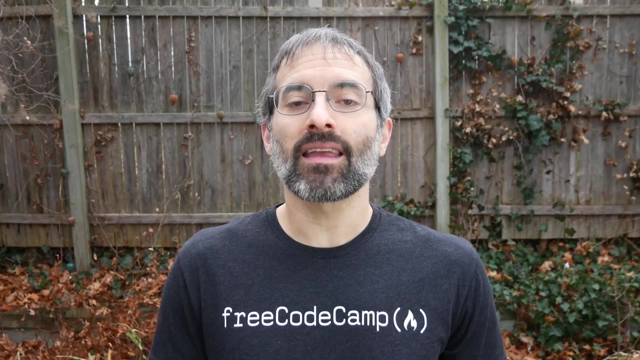 with the developer community are crucial for anyone who wants to be successful as a back-end developer. So here are some of the essential technologies you need to learn. You can watch a full, comprehensive course on each of these technologies right here on the FreeCodeCamporg YouTube channel as part of this back-end learning path. 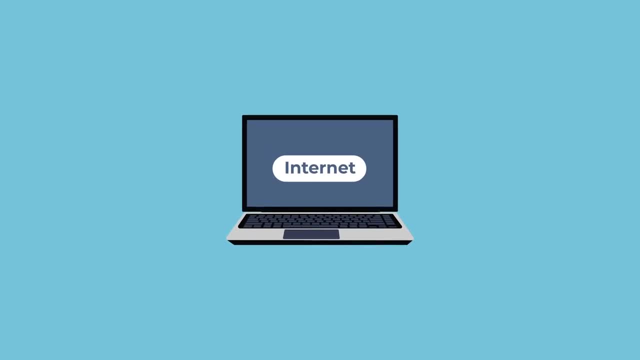 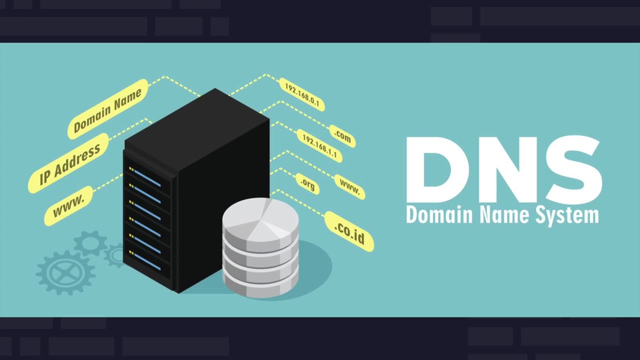 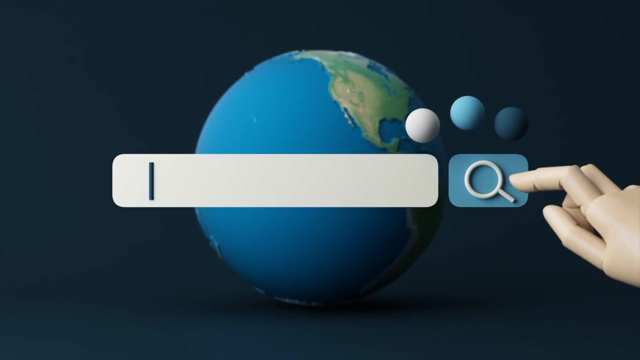 Understanding the basics of the internet is crucial for back-end developers. This includes knowledge of how data is transmitted over the internet, how DNS work and the roles of protocols such as HTTP and HTTPS. A solid grasp of these fundamentals allows back-end developers to build more efficient. 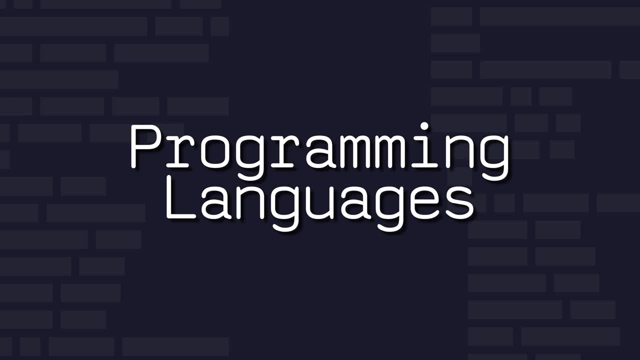 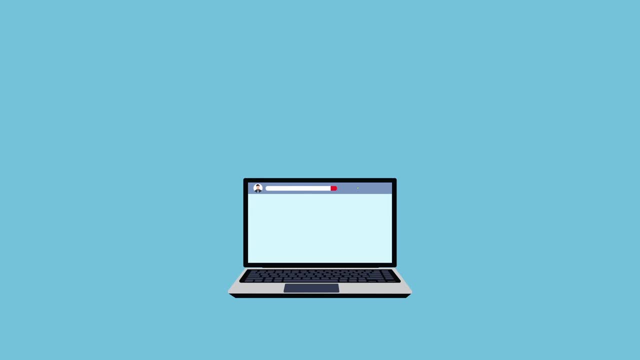 and secure applications. There are many programming languages used for back-end development. One is JavaScript. JavaScript was once confined to the browser, but now it's become one of the most popular languages for back-end development. Thanks to environment-based programming, it's now a popular language for back-end development. 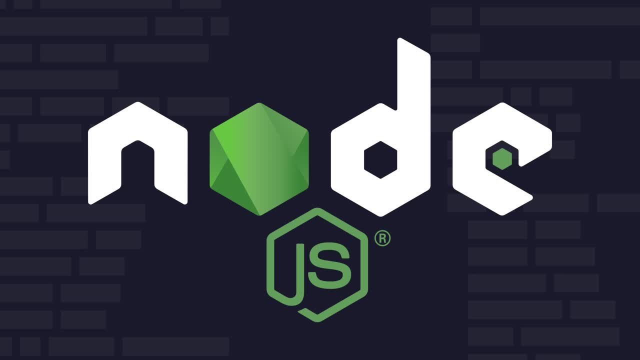 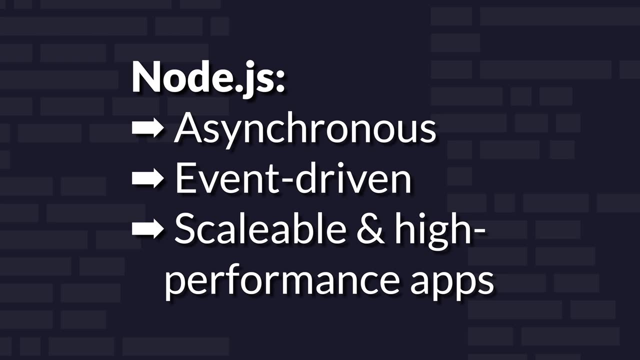 Thanks to environment-based programming, it's now a popular language for back-end development. It allows programmers to create different environments. like NodeJS, Its asynchronous nature and event-driven model make it suitable for developing scalable and high-performance applications. Python is renowned for its readability and efficiency, making it an excellent choice. 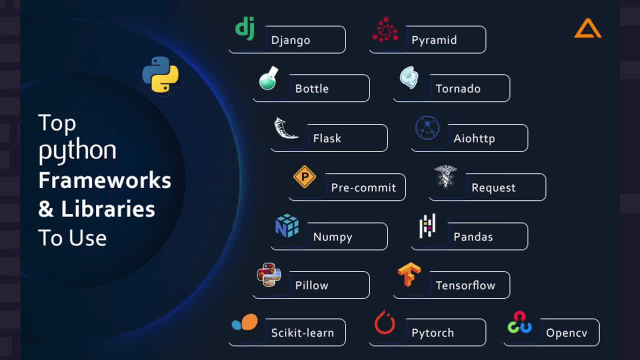 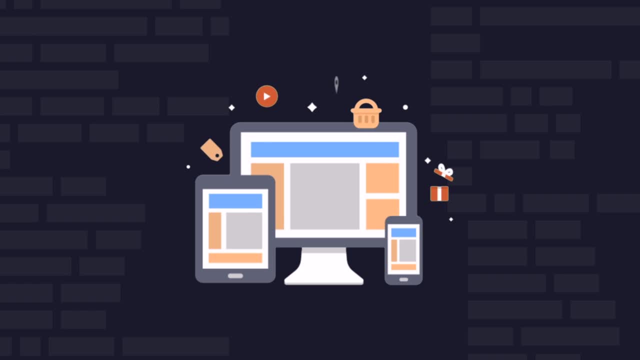 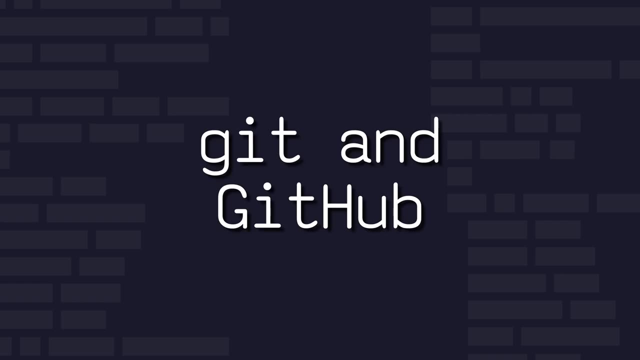 for back-end development. Its vast ecosystem of libraries and frameworks, such as Django and Flask, allow for rapid development of applications across various domains, And there are a lot of other commonly used programming languages, including Python. commonly used languages for back end development, such as PHP and Java. Git is a version control. 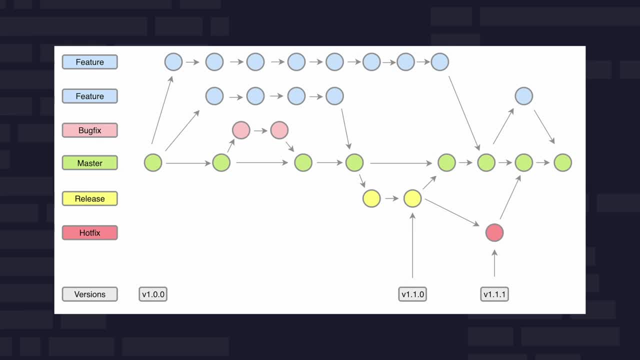 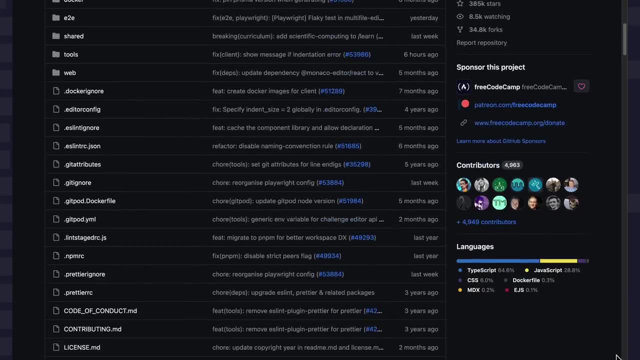 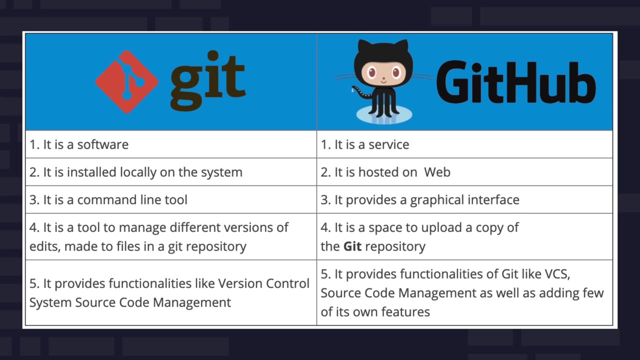 system that allows developers to track and manage changes to their code base. GitHub is a web based platform which leverages Git and enables developers to collaborate on projects, review code and manage changes. Understanding Git and GitHub is essential for back end developers to maintain. 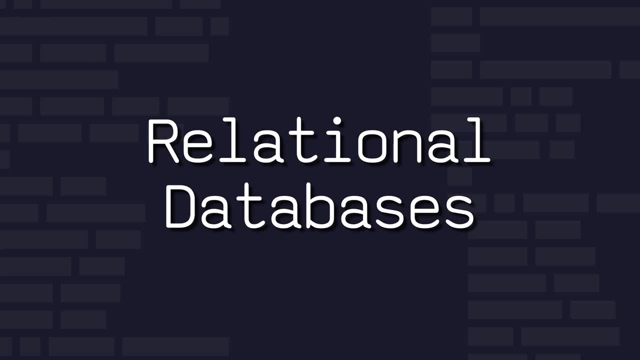 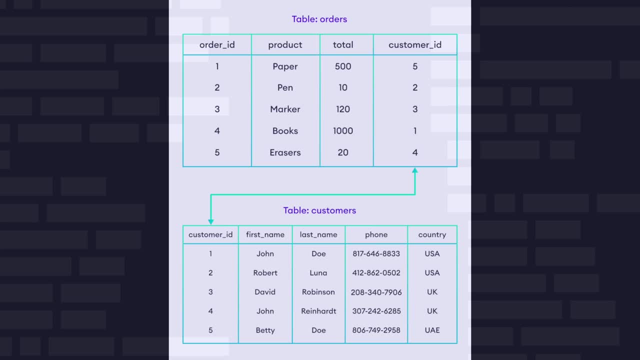 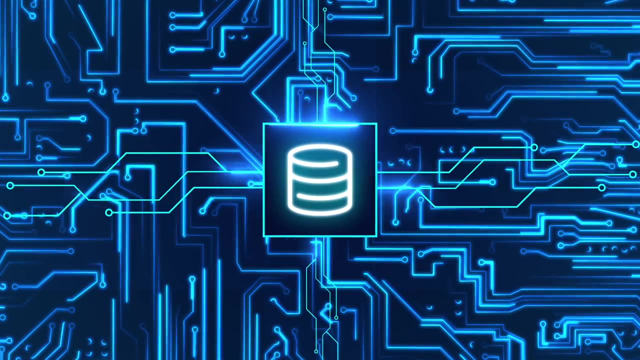 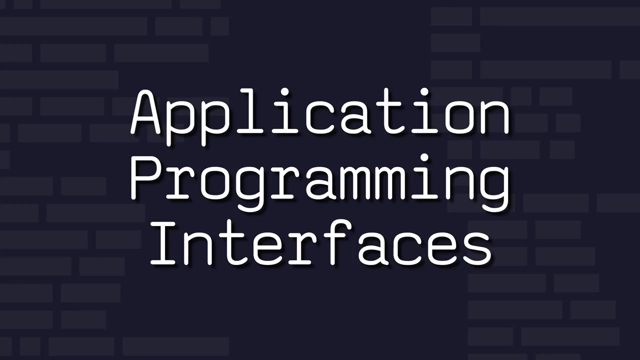 code integrity and collaborate effectively with others. relational databases store data and tables which can be linked to each other through relationships. Knowledge of relational database management systems like MySQL, PostgreSQL or Oracle is vital for back end developers to design, query and manage data efficiently, ensuring data integrity and performance Application. 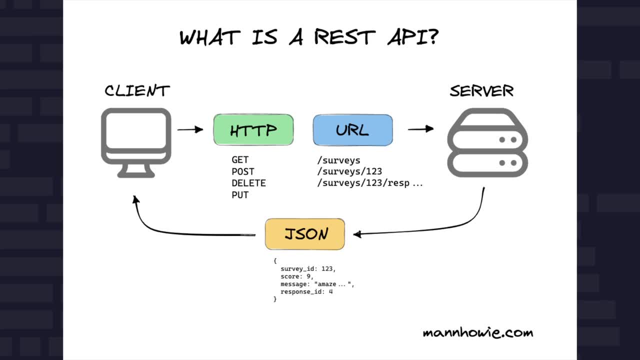 programming interfaces, or API's, allow different software systems to communicate with each other. So if you're looking for a way to manage your data efficiently, you can use GitHub, And if you're looking for a way to manage your data efficiently, you can use GitHub. Back end developers must. 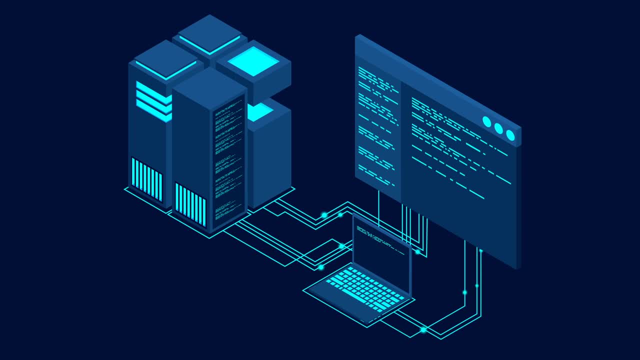 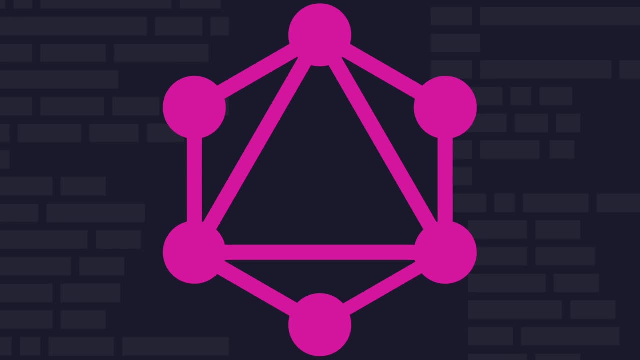 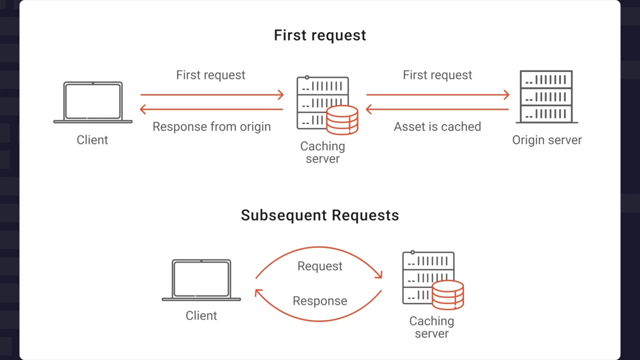 understand how to create, manage and document API's, as they enable the front end to interact with the back end, fetch data and perform operations. Knowledge of restful services and GraphQL is particularly valuable. caching is a technique to store copies of data in a temporary. 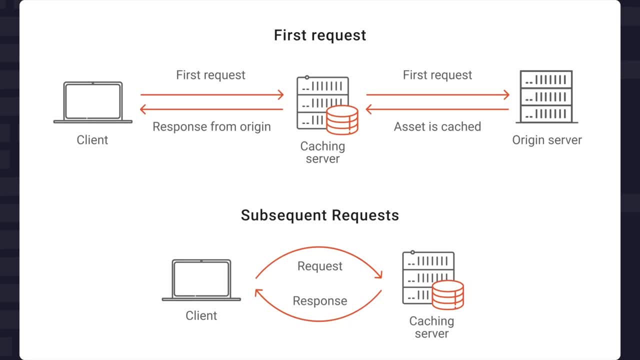 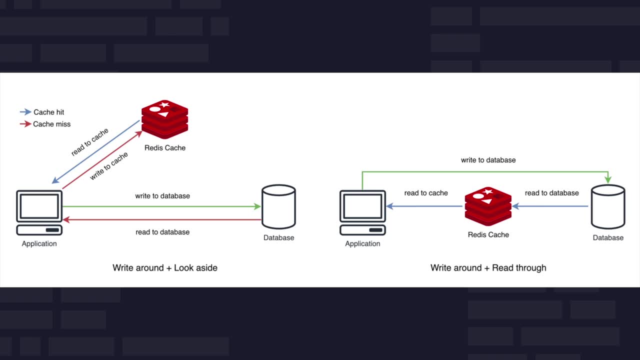 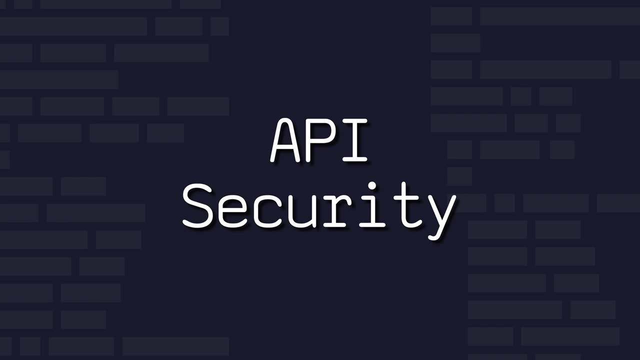 storage area which helps in reducing the load on the back end system, decreasing latency and improving the performance of web applications. Back end developers need to understand where and how to implement caching strategies effectively. API security is paramount to protect sensitive data and prevent unauthorized access. Back end developers. 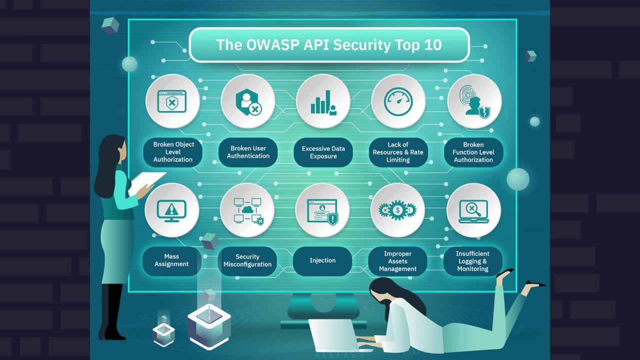 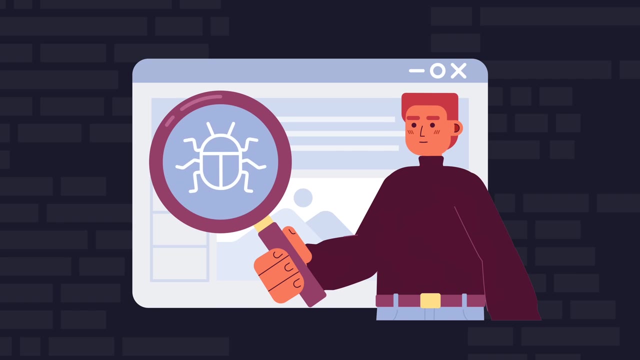 should be familiar with best practices such as implementing authentication, authorization, data encryption, rate limiting and regular security audits to safeguard the API's. Testing is critical to ensure the reliability and function ality of back end code. Developers should be proficient in various testing methodologies. 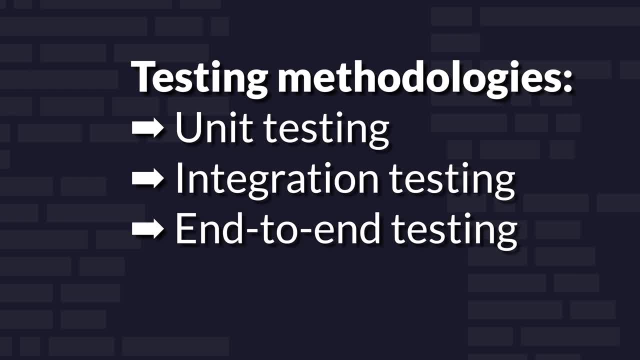 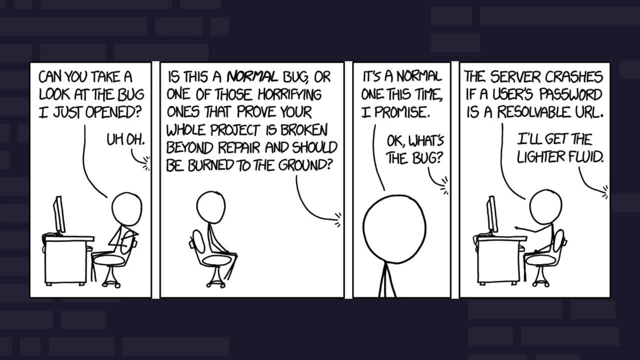 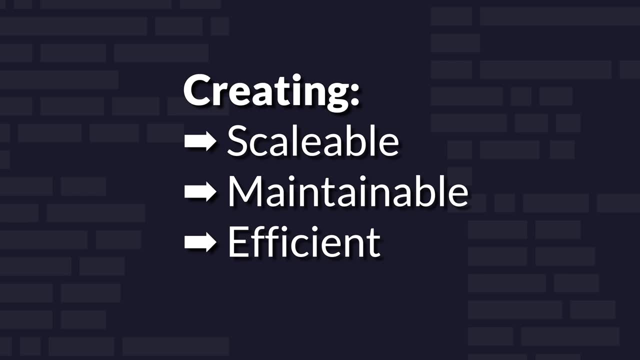 including unit testing, integration testing and end to end testing to detect and fix bugs, improve code quality and enhance the stability of the application. Understanding software design and architecture is crucial for creating scalable, maintainable and efficient back end systems. This includes knowledge of design patterns. 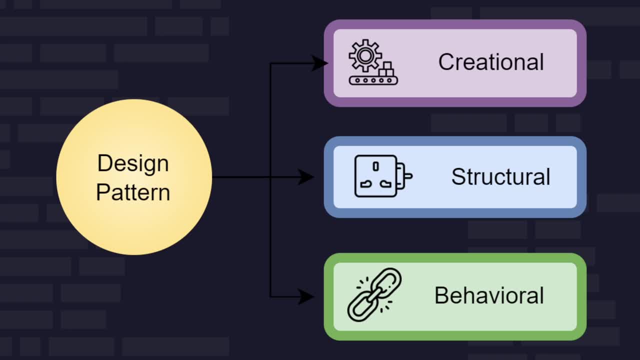 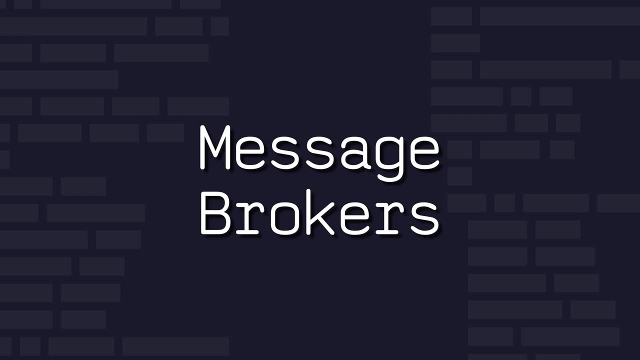 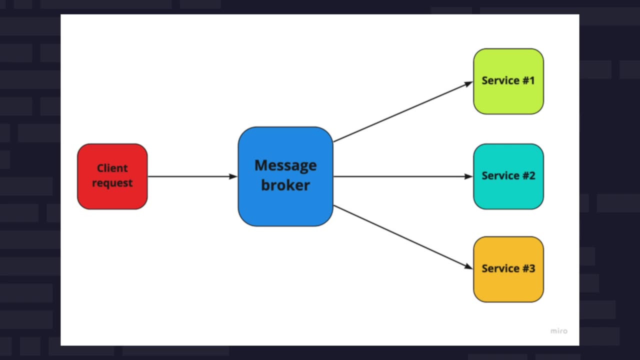 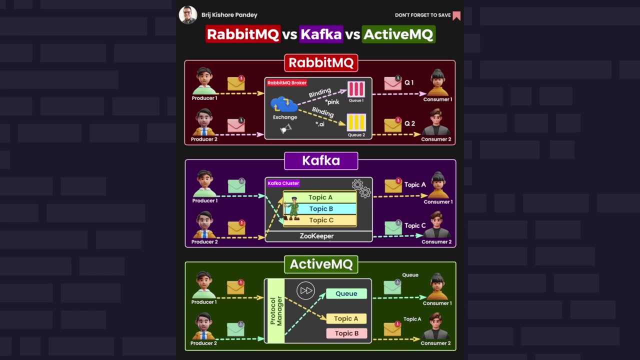 architectural styles and principles that guide the structuring of software systems for better performance and scalability. Message brokers like RabbitMQ and Kafka facilitate communication between different parts of an application through a reliable asynchronous messaging system. They're essential for building distributed systems enabling decoupling of application components. 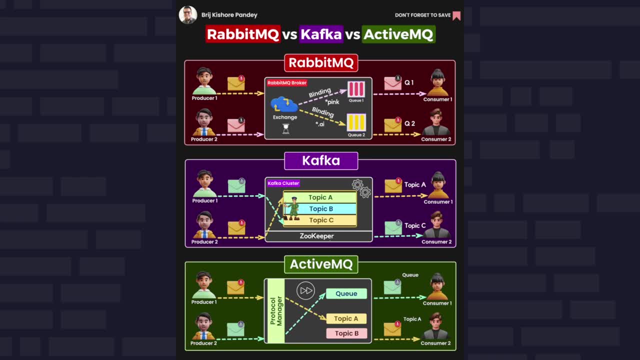 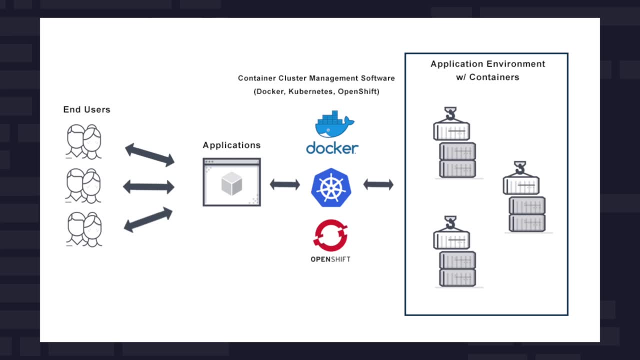 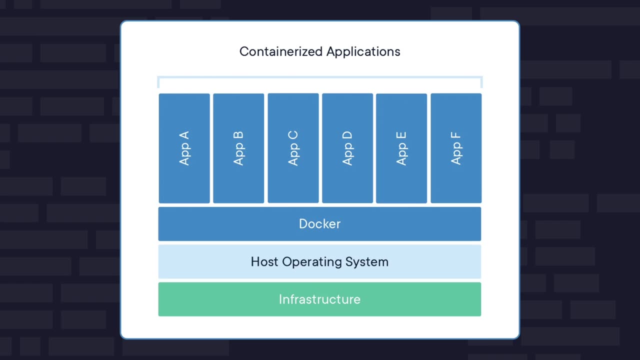 enhancing scalability and improving fault tolerance. Containerization technologies like Docker and Kubernetes are essential for creating, deploying and managing applications in an isolated, consistent and scalable environment. Docker packages applications into containers, while Kubernetes orchestrates these containers, managing their lifecycle across multiple 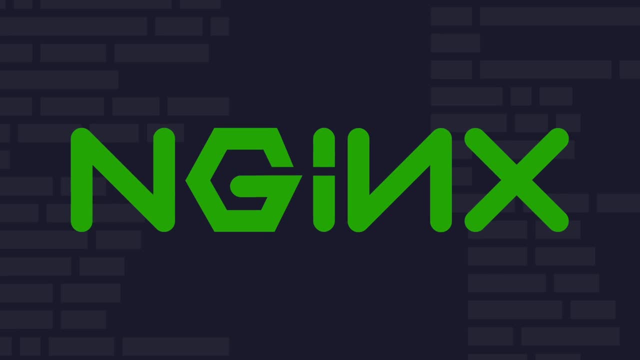 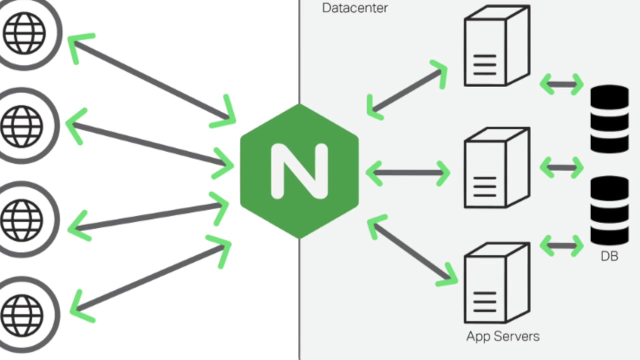 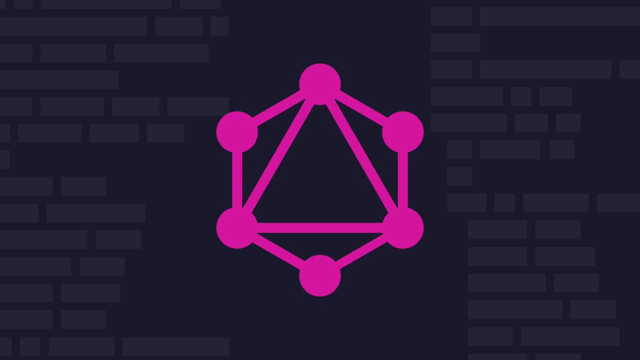 environments. Nginx is a popular web server known for its high performance, stability and efficient resource usage. Back end developers should understand how to configure Nginx to serve static files, proxy requests and handle load balancing, which is crucial for building scalable and reliable web applications. GraphQL is a query language for APIs that allows 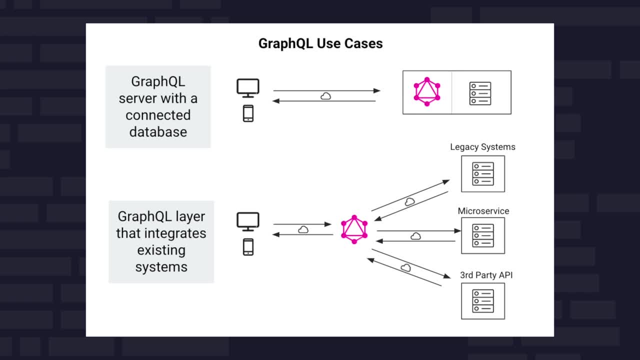 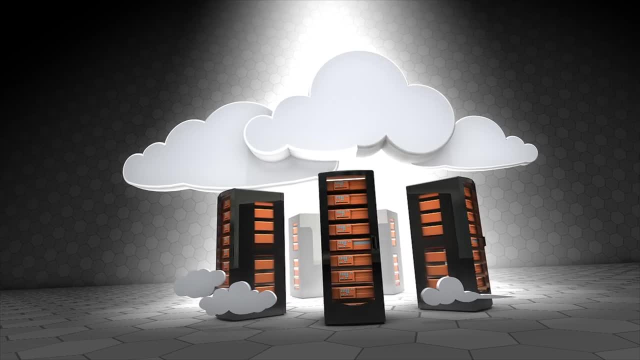 clients to request exactly the data they need, making it an efficient alternative to traditional REST APIs. Back end developers should understand how to implement GraphQL servers to provide flexible and efficient data access. MongoDB is a very well-known and well-known web server. It's 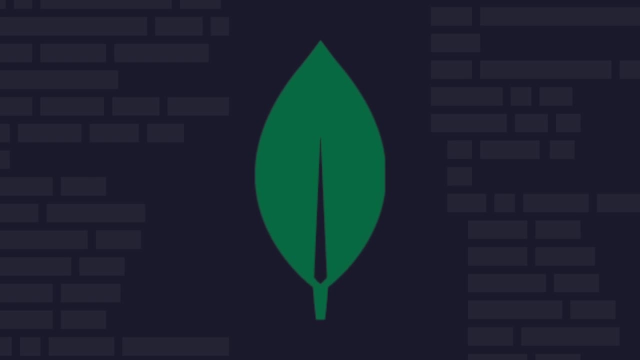 one of the most well-known and well-known web servers in the world. MongoDB is a very well-known and well-known web server. MongoDB is a very well-known and well-known web server. MongoDB is a NoSQL database that stores data in flexible JSON like documents, allowing for fluid data models. 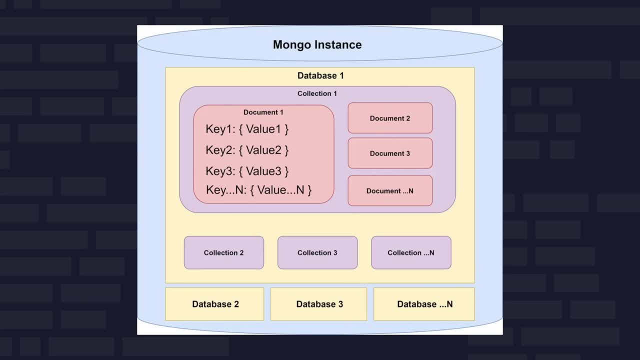 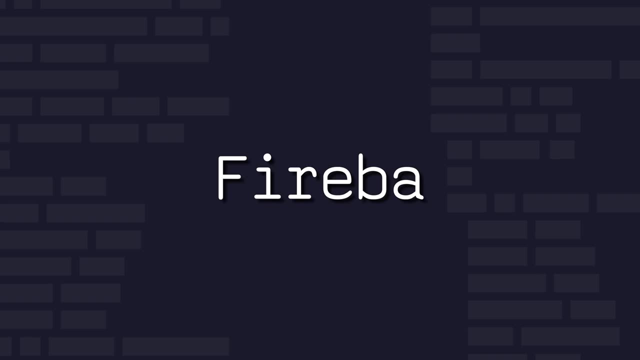 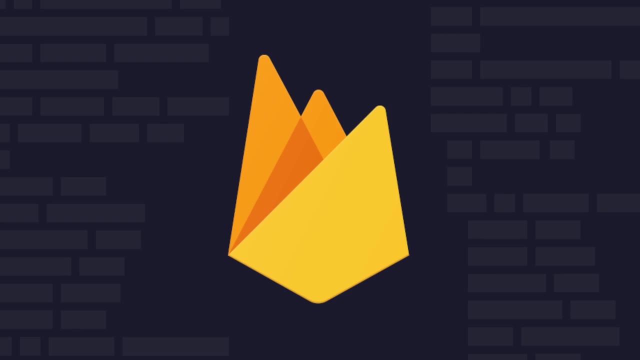 and rapid development. It's particularly useful for applications that require scalability, fast querying and the ability to handle a variety of data types. Firebase provides a comprehensive suite of tools for building web and mobile applications, including real time databases, authentication and hosting. It's favored for rapid development and. 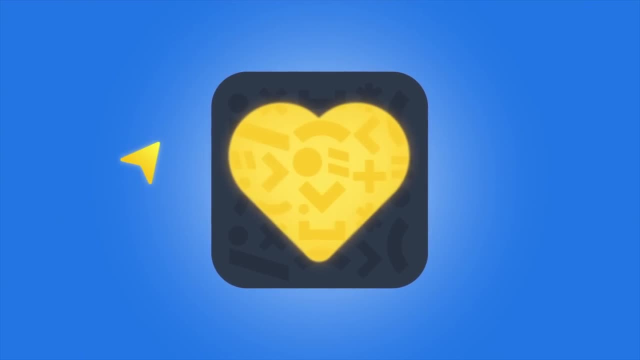 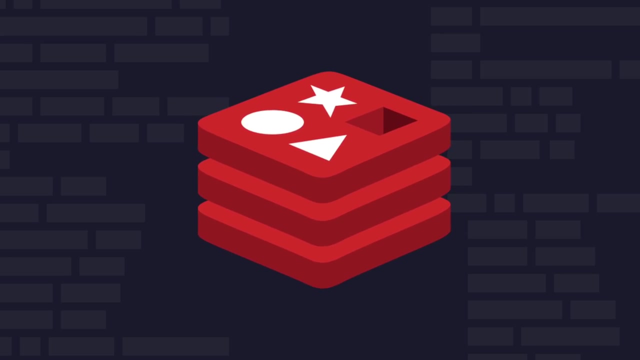 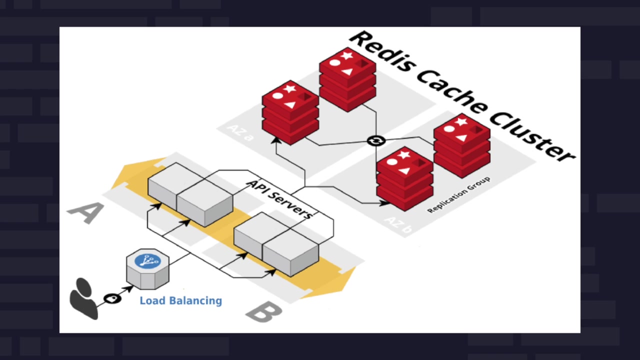 its ability to scale automatically, making it a popular choice for startups and agile projects. Redis is an in memory data structure store used as a database cache and message broker. It's high performance and support for various data structures, such as strings, hashes and lists, make it invaluable for scenarios requiring fast access to. 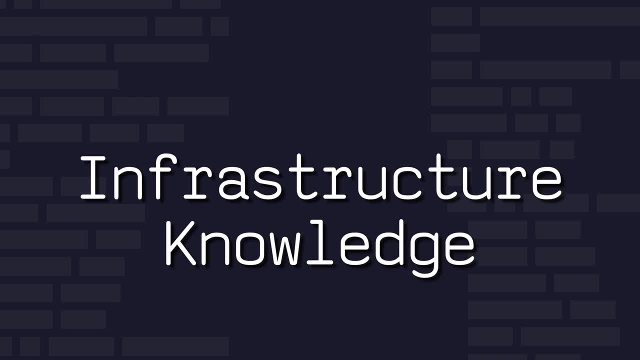 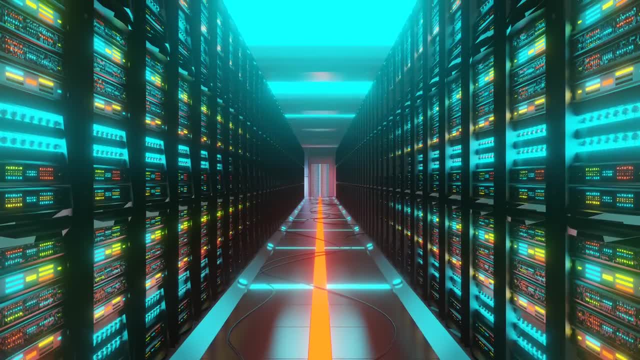 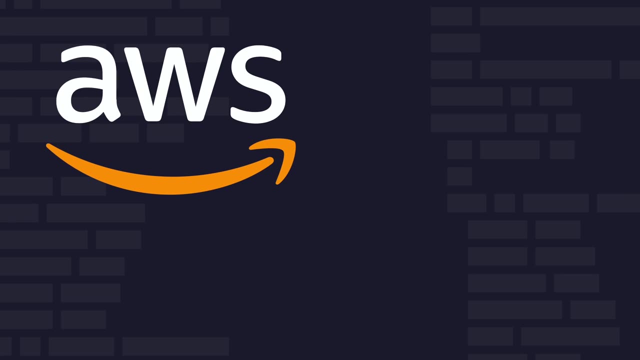 data such as caching. Understanding the underlying infrastructure is crucial for back end developers. This includes knowledge of servers, networks, cloud services and how they interconnect to deliver applications, Familiarity with cloud providers like AWS, Azure or Google Cloud, and services like virtual machines, container orchestration. and serverless computing can significantly enhance the efficiency and scalability of applications. Back end development is a constantly shifting and evolving landscape, with new technologies and emerging and best practices being refined regularly. Keeping up with these changes and remaining adaptable is essential in this field. This roadmap lays a solid foundation. 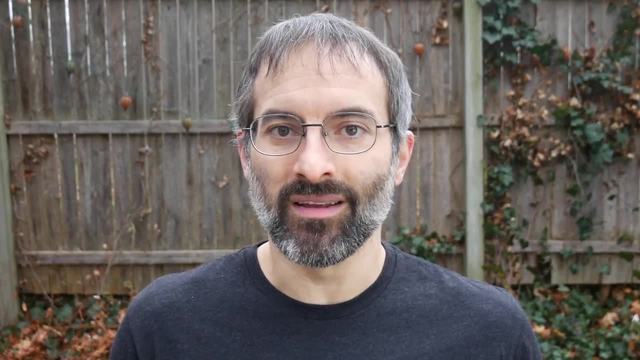 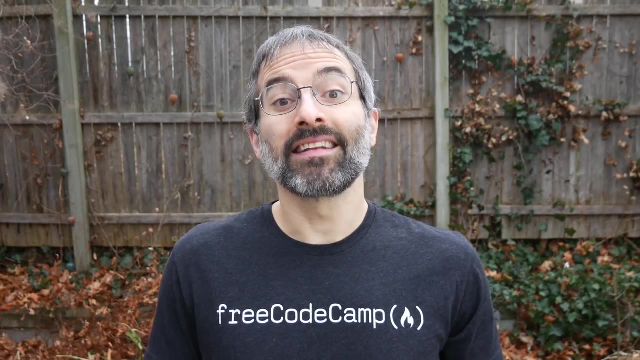 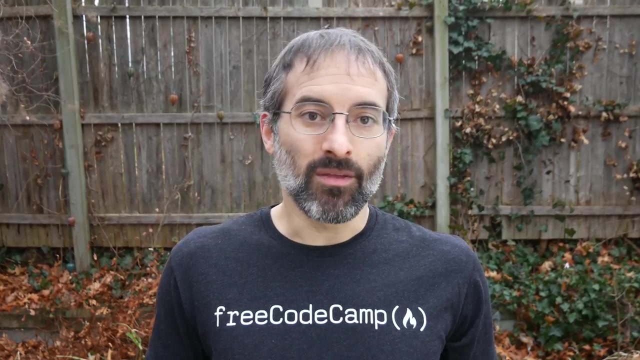 but the journey of learning and growth. in back end development is continuous. There are numerous popular tools and frameworks not included in this roadmap. However, starting somewhere is important and the technologies I've mentioned are an excellent beginning point. Engage actively with the developer community. experiment with emerging tools. 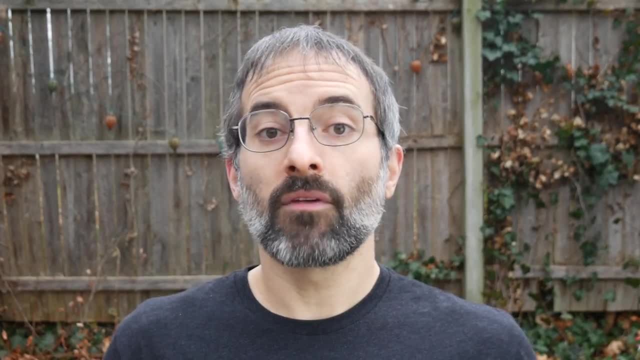 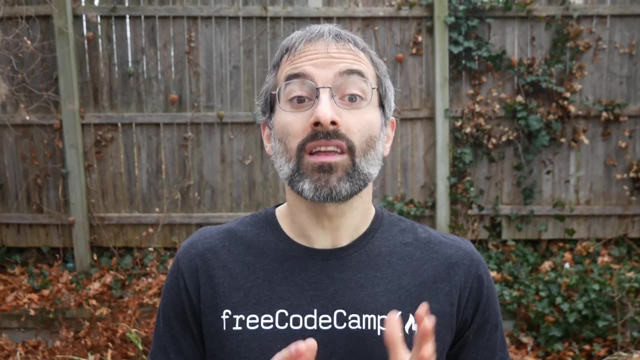 and always aim for excellence. The realm of back end development has many opportunities. With the right set of skills and knowledge, you can develop powerful, efficient and secure back end systems. So good luck on your learning journey.